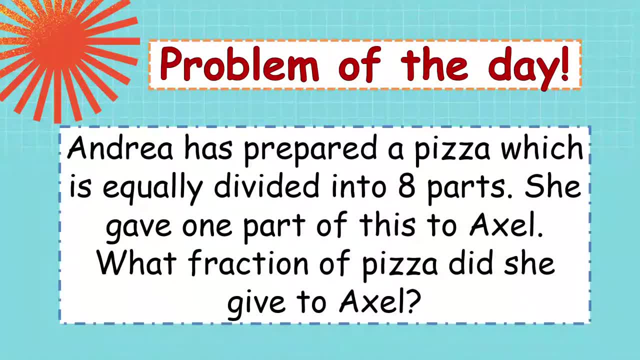 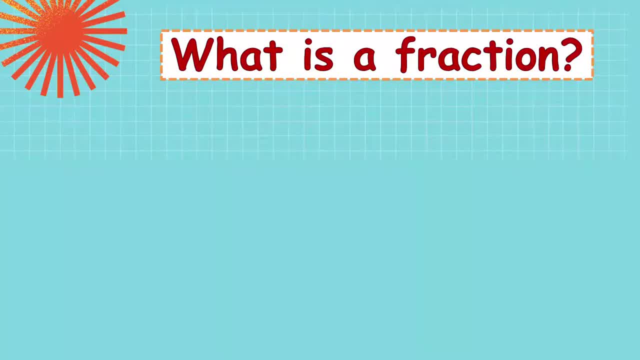 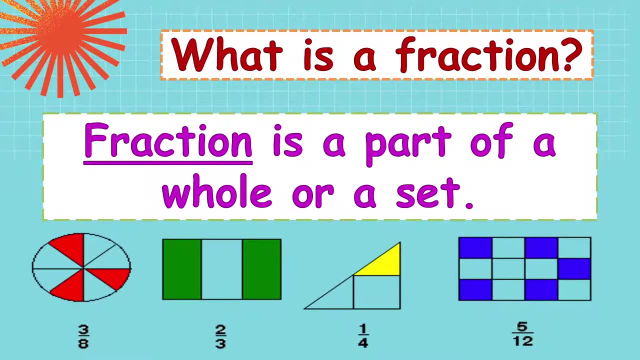 All right, so let's go back to this problem later. Let's discuss first fractions. Okay, what is a fraction? Fraction is a part of a whole or a set, For example. look at the circle. The circle is divided into eight equal parts. Okay, and look. 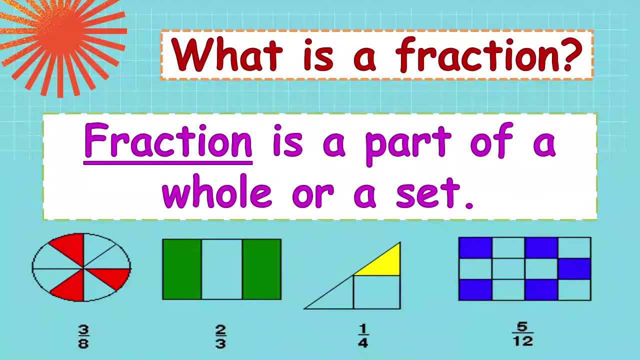 how many colored parts are there? Three, So the name of the colored part is: the fraction is three parts. Next, how many parts are there? Look at the rectangle. the second one: Yes, there are three equal parts, And then two parts are colored. So the name of the fraction is two-thirds. Okay, 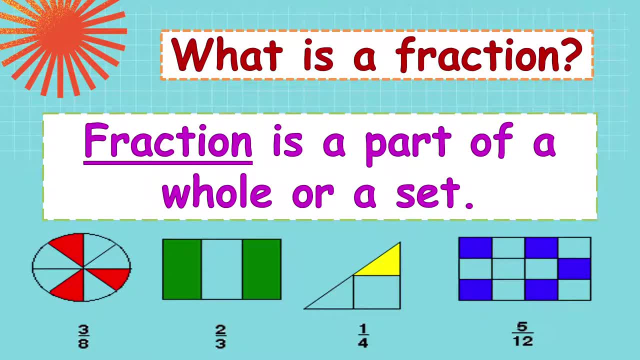 all right, That means two colored parts out of three parts. All right. next, look at the triangle. The triangle. as you can see, there are three, But you put together two triangles, small triangles. you can form a small rectangle. okay, The shape looks like a rectangle. All right, Okay, so one part. 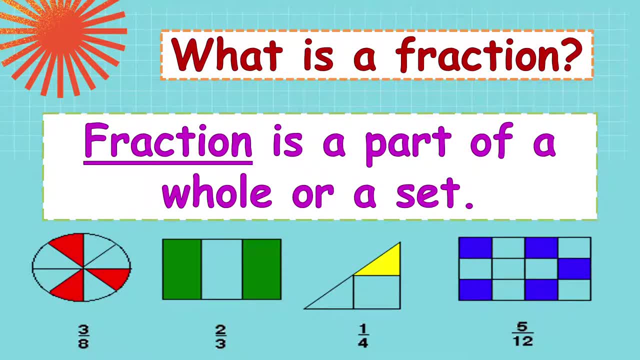 is colored yellow, So that represents one-fourth, Okay. next the rectangle is divided into twelve equal parts. And then how many parts are colored blue? Five. So the name of the fraction is of the colored part: is five twelves, okay, so let's go back now to the problem. 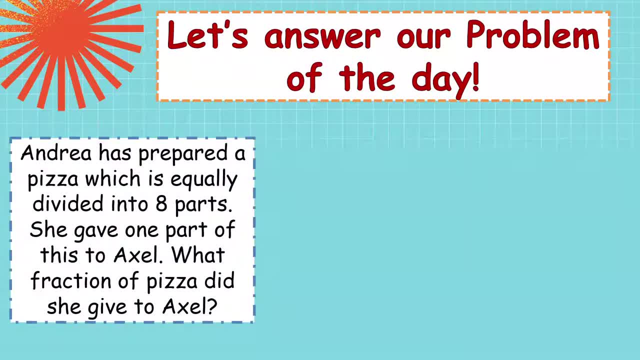 let's answer the problem of the day. so how many pizza did andrea buy? yes, there is only one whole pizza, but she divided it equally into eight equal parts. okay, and then, all right, that eight equal parts, that will be our denominator. okay, that's the number that we're. 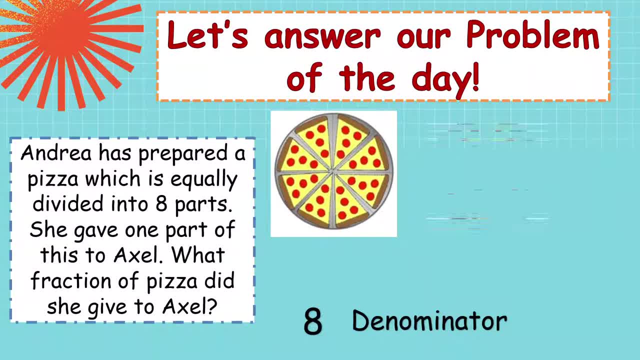 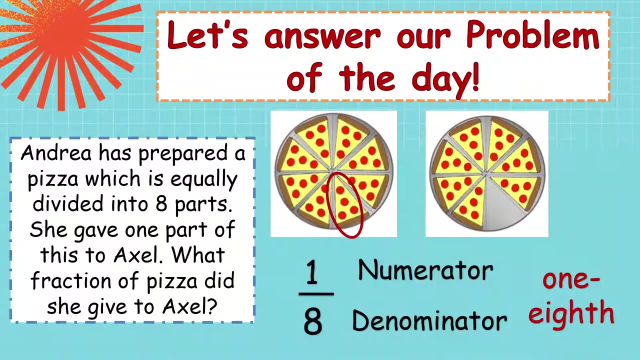 going to write at the bottom and look, one pizza is missing because that one pizza was given to axel. so we can say one. that is our numerator. so we gave, or andrea gave, one to axel. so we can say that the fraction of pizza that andrea give to axel is 1: 8th. one pizza, one piece out of the eight parts. 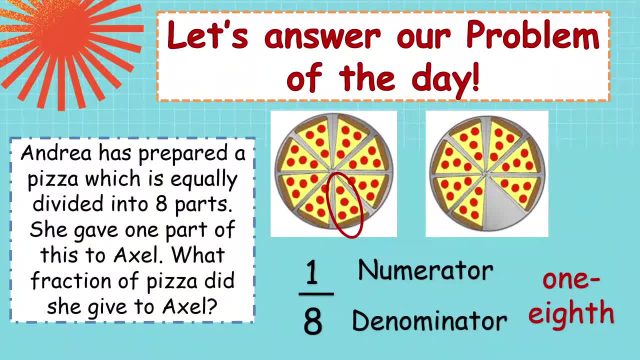 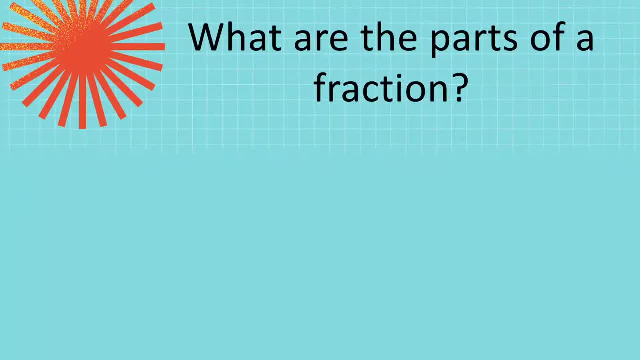 eight equal pizzas. okay, all right, so it's one if that's the answer, all right. so let's go back. what are the parts of a fraction again? so there, for example, we have 1- 5th. there are five questions, and then you missed to answer one item. okay, so. 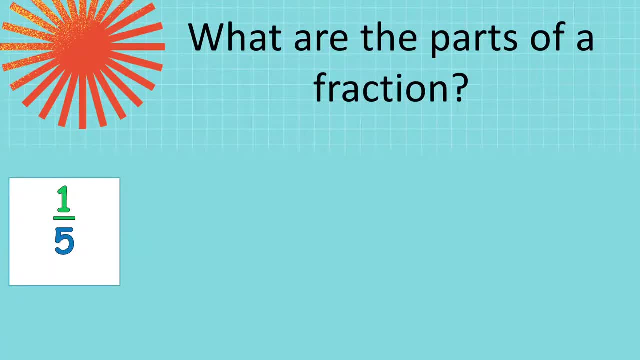 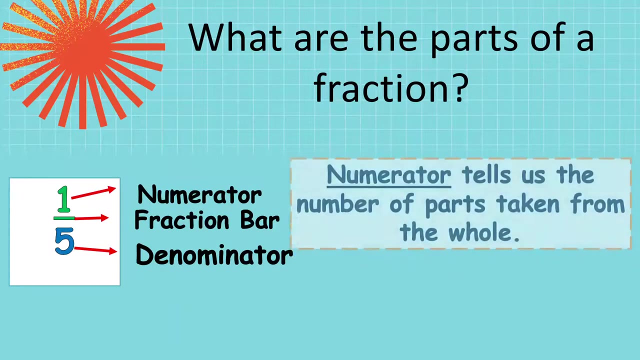 the fraction of the answer of the items that you miss is one fifth. so one is the numerator, five is the denominator and that line between one and five is our fraction bar. okay, so let's define numerator. numerator tells us the number of parts taken from the whole. 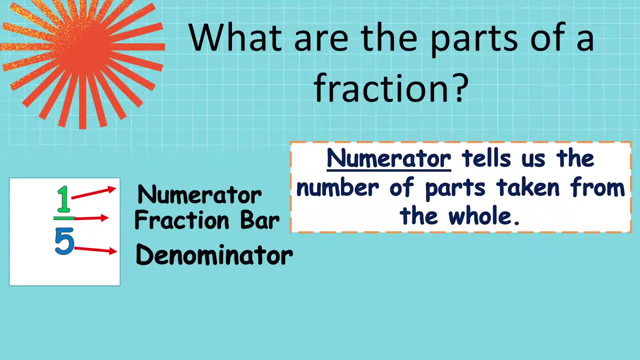 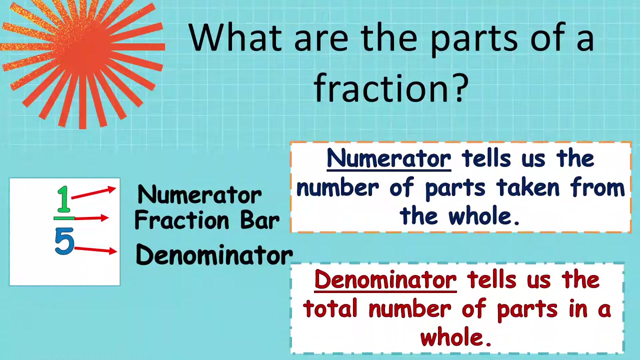 Alright, just remember the pizza We took one. that's the numerator. Or, in this example, there are five questions. You missed one item to answer That one item that you missed is our numerator And the denominator tells us the total number of parts in the whole. So there are five questions. Five is the denominator. There are eight equal parts in the pizza, So eight is the denominator. 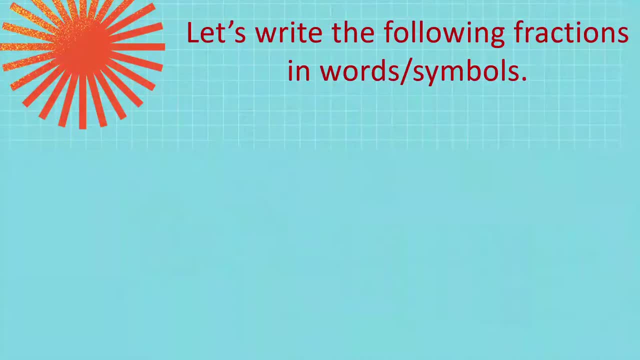 All right, Okay, so let's practice. Let's write the following fractions in words and in symbols. So that is written in words, So we're going to write that in symbols. So one-sixth, So one, and then the fraction bar, and then sixth, the denominator One-fourth. Okay, that's how we write one-fourth And then one-third. 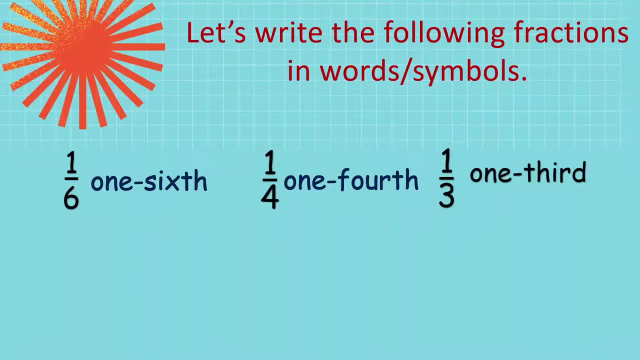 So, children, what do you notice when you write the denominator? Very good, It's written in like an ordinal number: right, Sixth with the th, fourth with the th, third with the rd. get the position right, Remember ordinal numbers. So we write it that way. 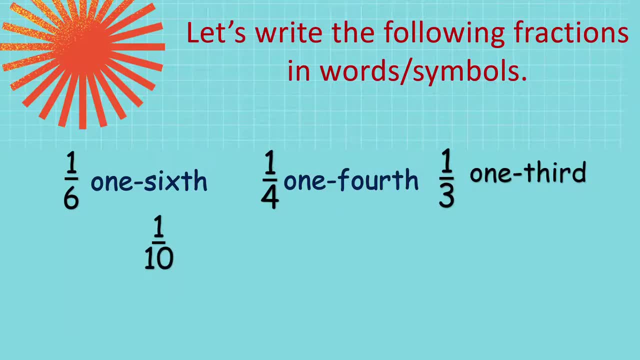 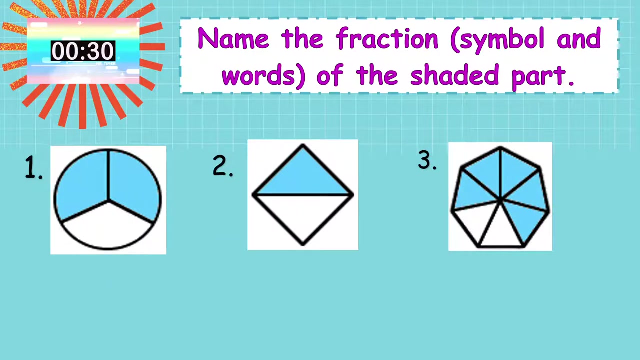 Okay. so let's have another one. So this time it's written in symbol. We're going to write it in words. So how do we write one-tenth? Okay, it's how we write one-tenth, one-ninth and one-half. Okay, very good. Now it's your turn. I'll give you 30 seconds to think. Okay, to write the fraction in symbol and in words: Okay, of the shaded part. Are you ready? Okay, go. 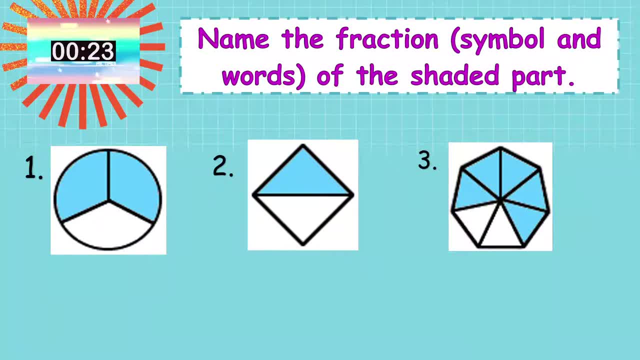 All right time is up. Very good, Show me your answer, Or check your answer, if it's correct. Okay for number one: Yes, there are two shaded parts, So two and then three. That's the denominator. So we say two-thirds with s because there are more than one right Okay. next, Yes, one-half Okay, very good. And then next, Yes, five-sevenths. 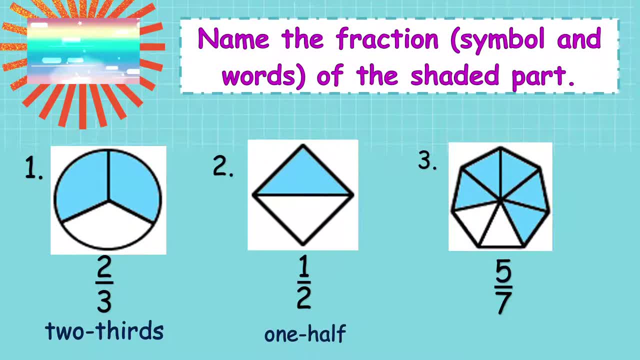 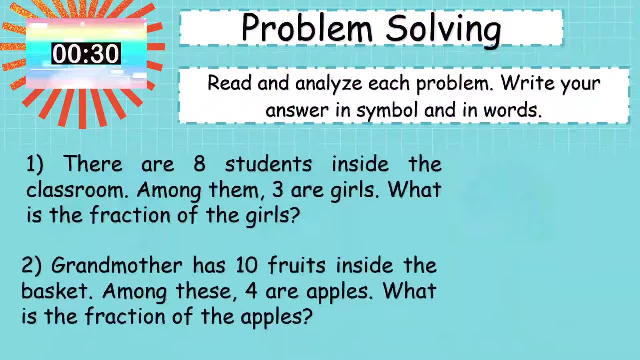 Five shaded parts, Okay, and then there are seven equal parts. So five-sevenths, Yay. very good, All right, Now can you answer these problems? Two problems, Okay. I'll give you 30 seconds again. Ready Go. 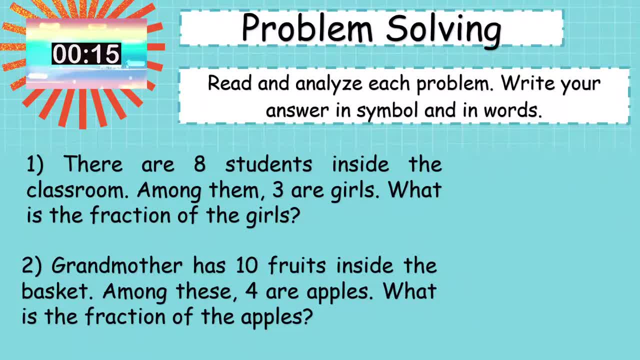 All right, let's see Number one. there are eight students inside the classroom. Among them, three are girls. What is the fraction? What is the fraction of the girls? Okay, All right. Yes, there are three girls, So three out of eight. So we say three-eighths, Okay, good job. Next, Grandmother has ten fruits inside the basket. Among these four are apples. What is the fraction of the apples?